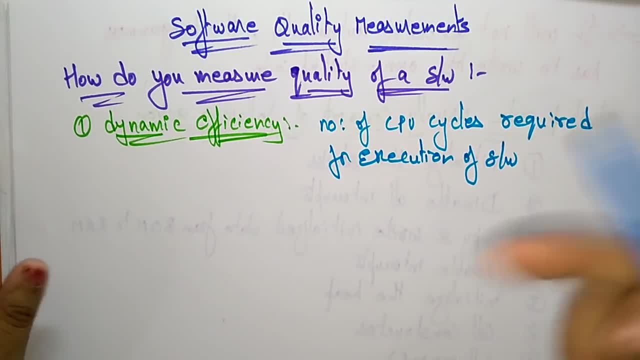 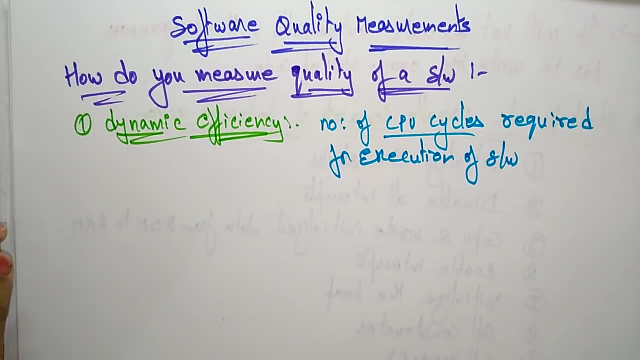 So that you call it as a dynamic efficiency. The dynamic efficiency of a software can be identified by with the help of number of cycles That required for execution of a software. If you want to perform some operation, so how many CPU cycles are required? 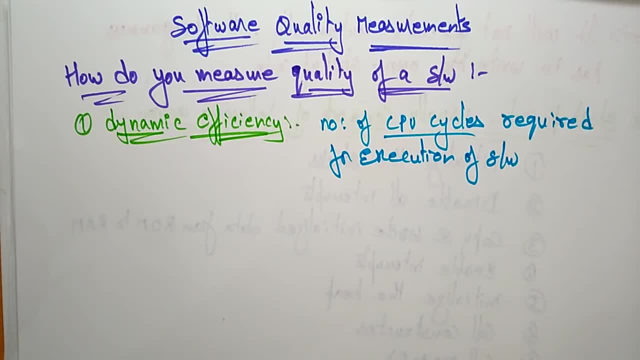 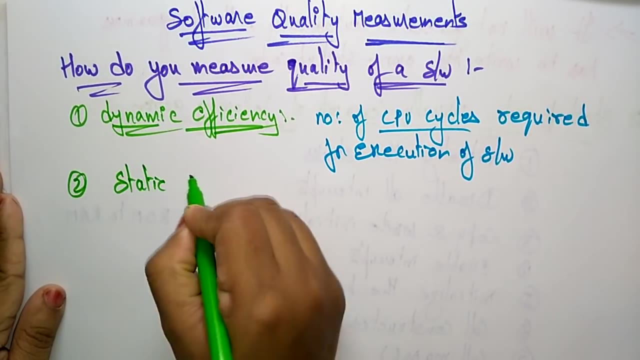 So if it requires the less CPU cycles within less CPU cycles, if the task is going to be completed, then you can say your software is highly qualified, which is supporting the dynamic efficiency. So in the next is a static efficiency: Static efficiency. 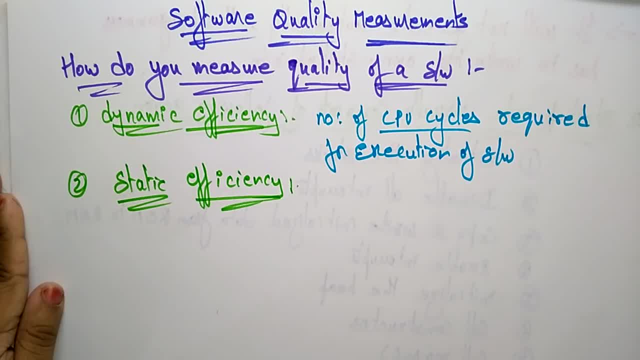 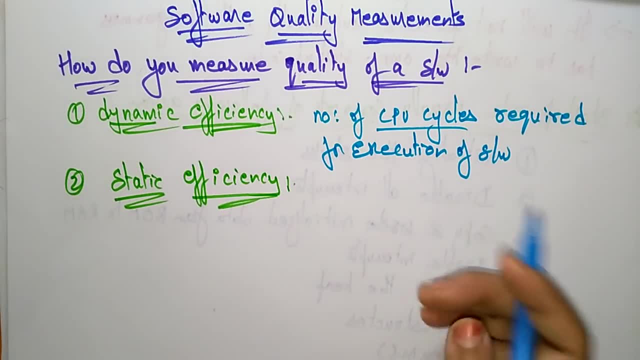 Static efficiency. So not only that, In the dynamic efficiency, you have to consider the static efficiency also. The static efficiency can be identified by using number of bits required, with the help of number of bytes required to execute the task. So how many bytes are required? 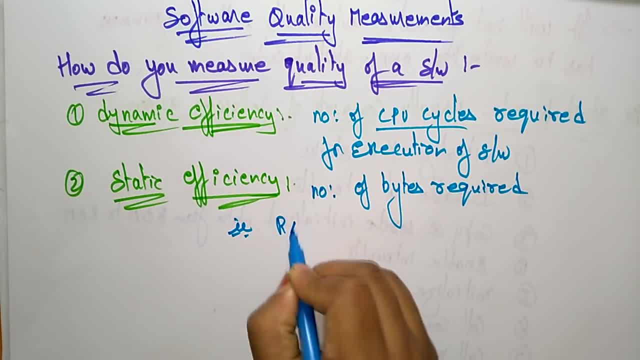 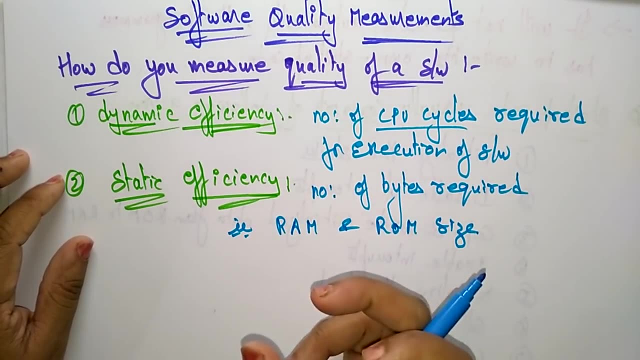 So that is a RAM and ROM size. Simply you can say the RAM and ROM size. So RAM always Stores the, determines the global variables and runtime stack. So RAM depends upon the completely holds the global variables and runtime stack, Whereas a ROM determines the fixed constants on a program code. 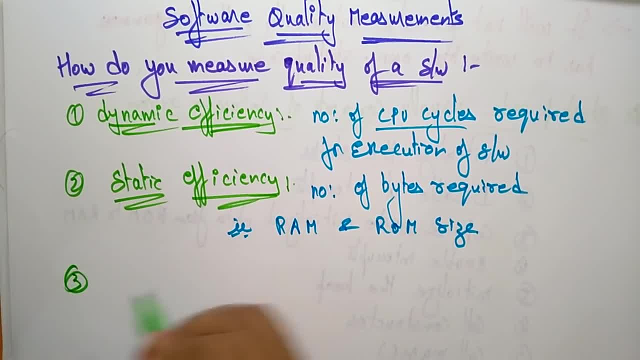 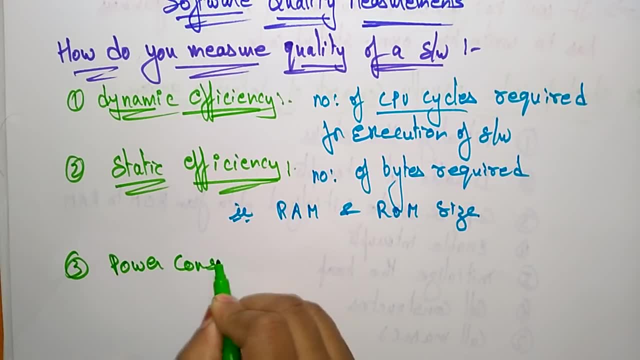 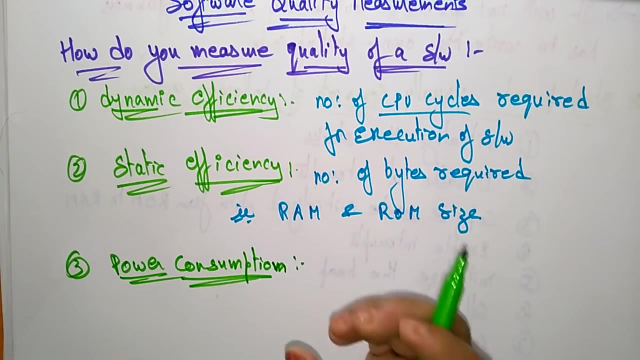 And the next thing is power consumption. So you can measure the software with the help of power consumption. So how much power it is going to be consumed to execute the task, Your embedded system is going to be consumed, So power consumption is an another issue. 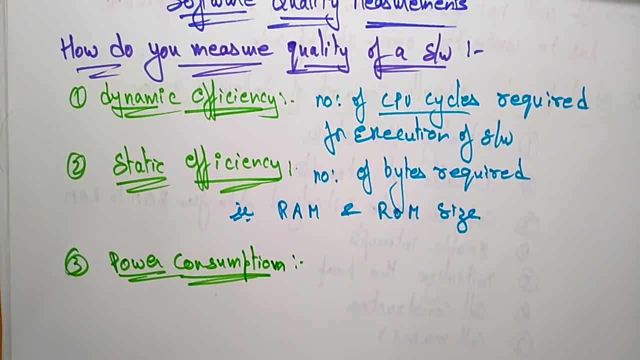 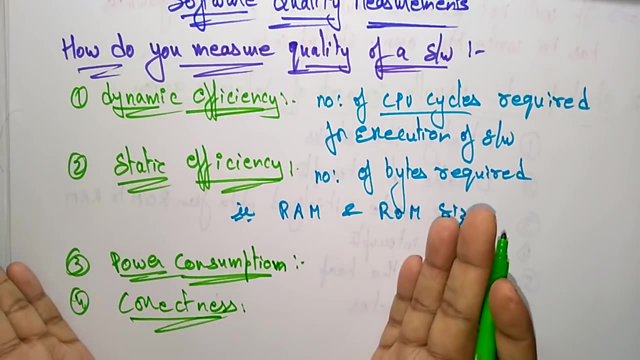 So if you, if you are designing any product, any controller, you have to think about the power consumption. Next is the correctness. How much correctness it is giving the correct output? here It's completely maintaining and reusing the software. So is there is a chance of reusing your product if it is not working on that particular task? 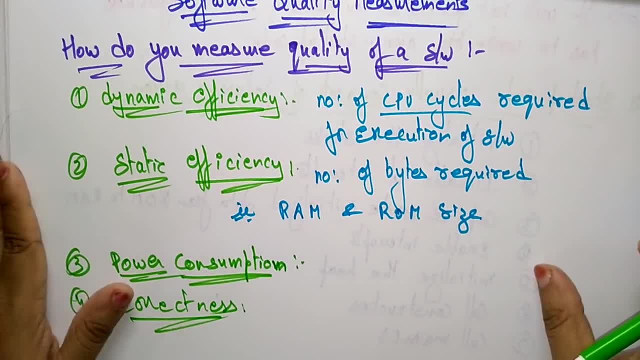 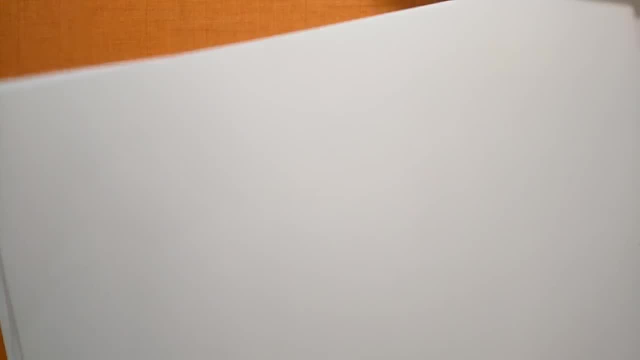